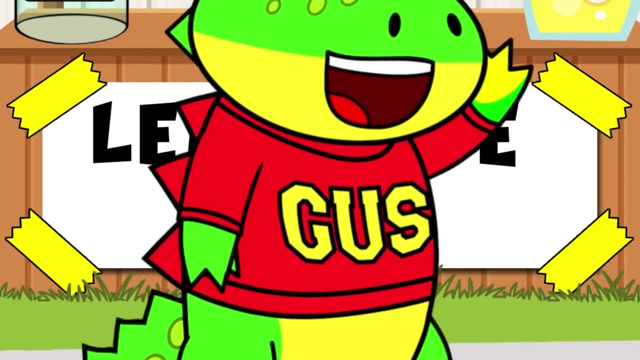 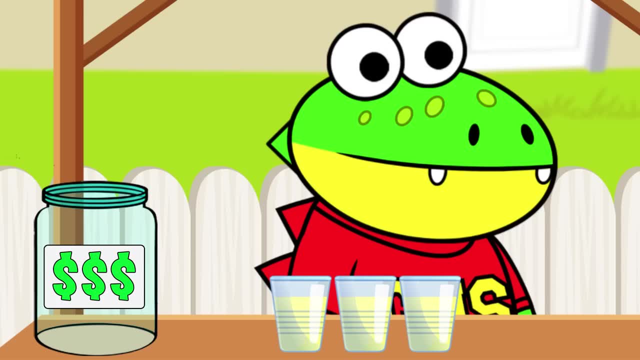 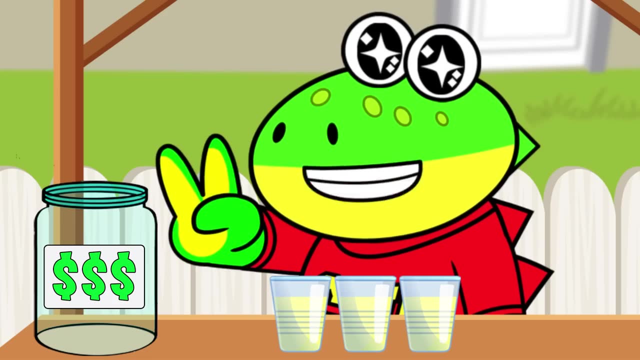 Hiya little gators, I'm going to sell some lemonade. Get your lemonade Only 50 cents. Whoa, Where did all these customers come from? Looks like we're in business Vegas. your lemonade stand is really cool. I'll take one cup, please. 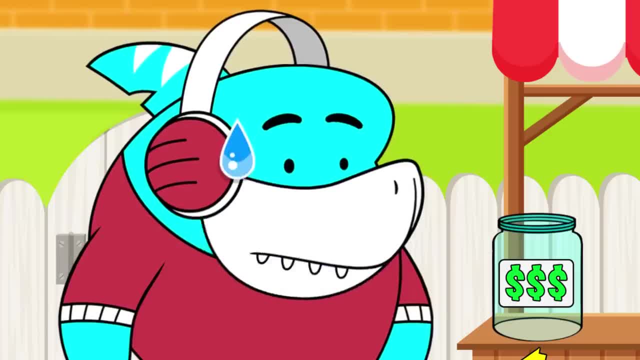 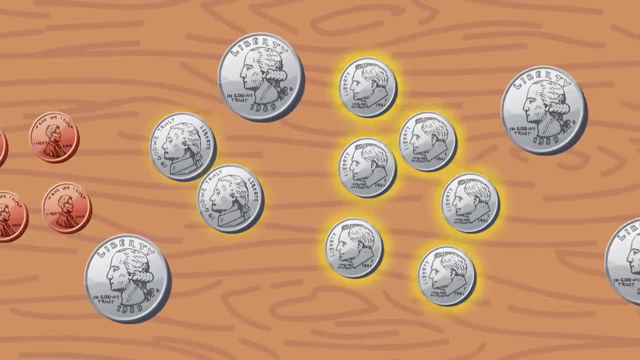 Thanks, Gil, That'll be 50 cents. Oh, dude, I only have one dollar. I don't mind waiting for my change. Uh, there are pennies, nickels, dimes, Oh, my, Oh, I don't know which coins to use, little gators. 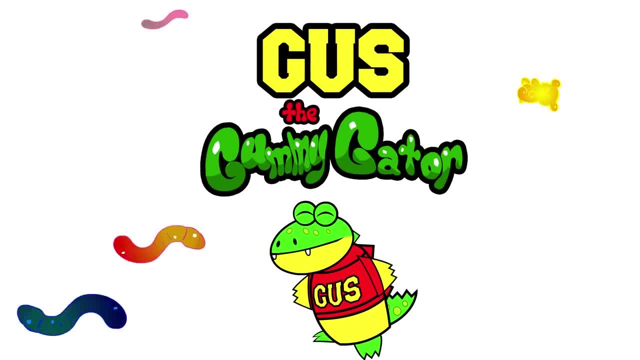 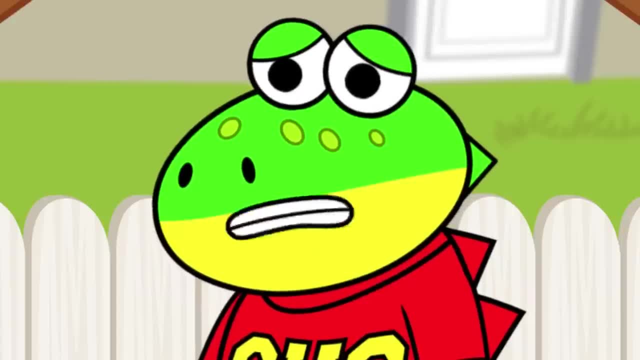 Gimme that yummy gummy. I'm Gus the Gummy Gator. Hi Shug, How's everything going with your lemonade stand? Well, Gil gave me a dollar, but I'm not sure how much change to give back. 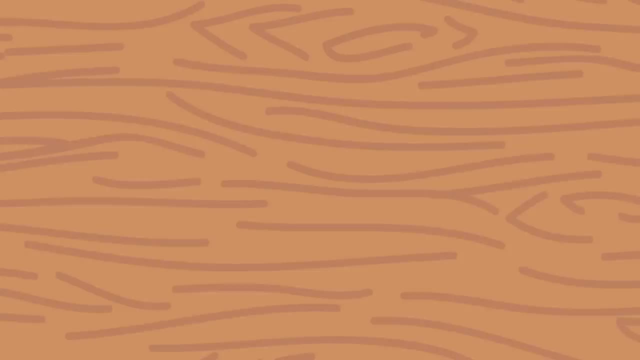 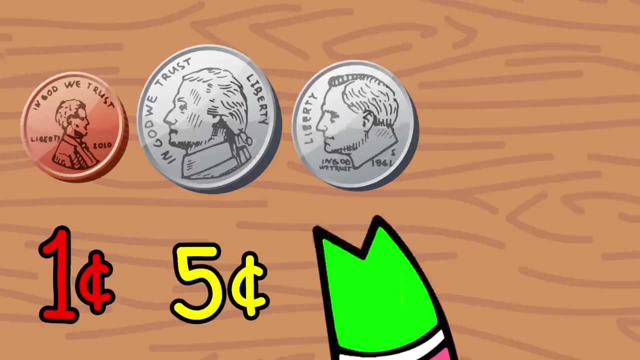 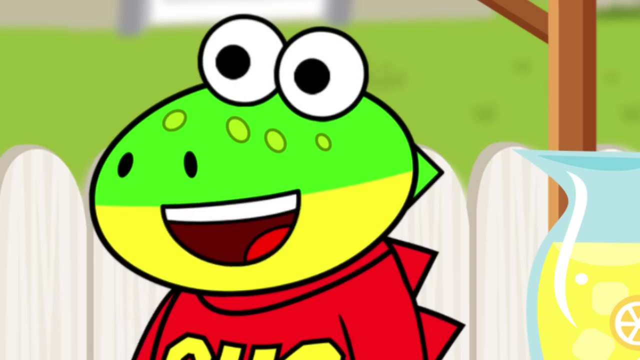 No problem, Gus, I'll help you figure it out. First. a penny equals one cent, a nickel equals five cents, a dime equals ten cents and a quarter equals 25 cents. Got it. But how much does a dollar equal? 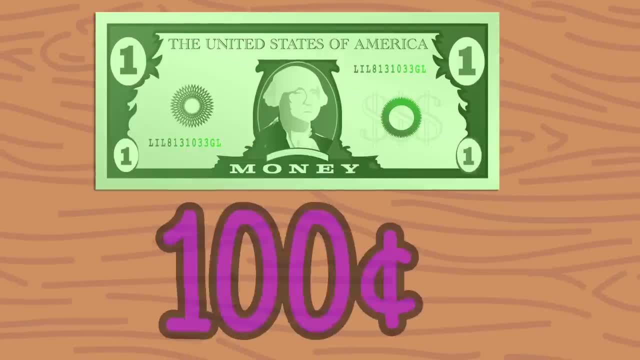 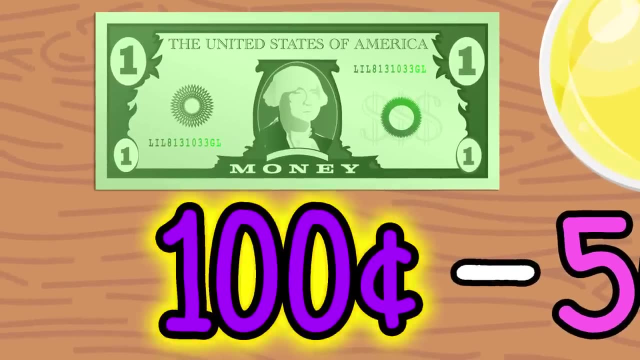 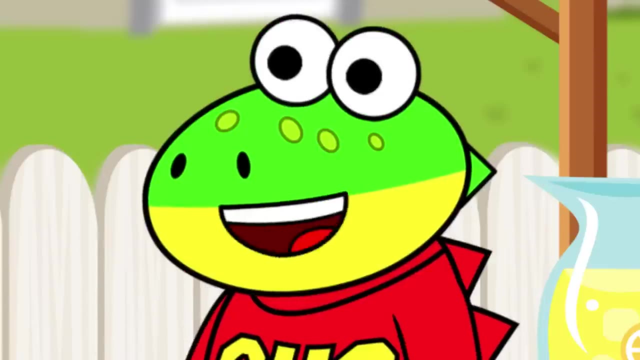 Good question. A dollar equals 100 cents. So if the lemonade is 50 cents and Gil gives you 100 cents, you need to give him 50 cents back. Oh, So that means I could give him two quarters back. 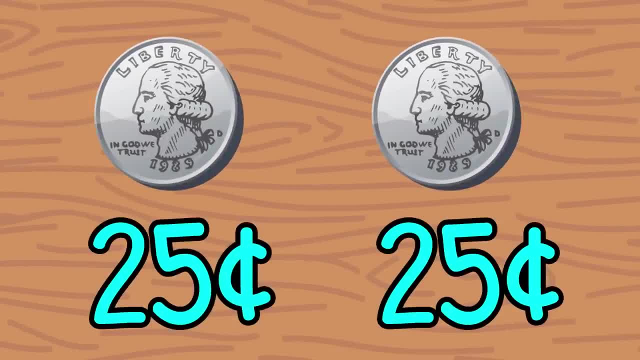 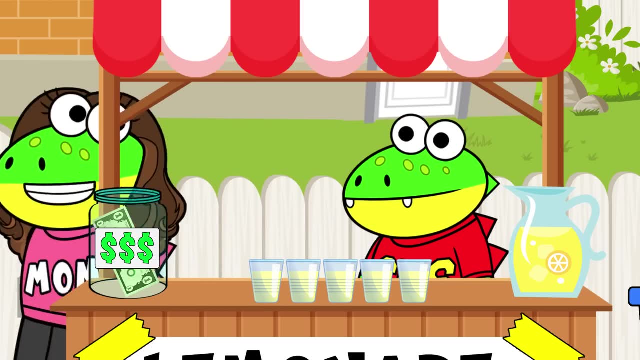 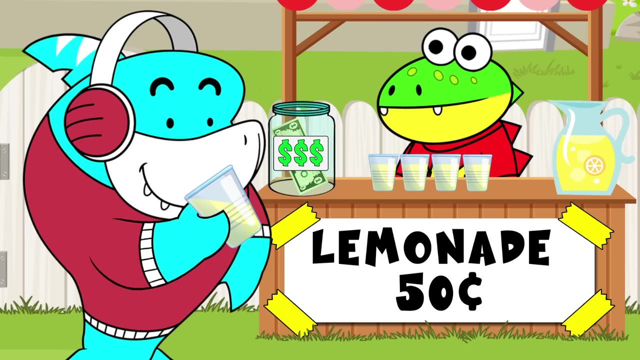 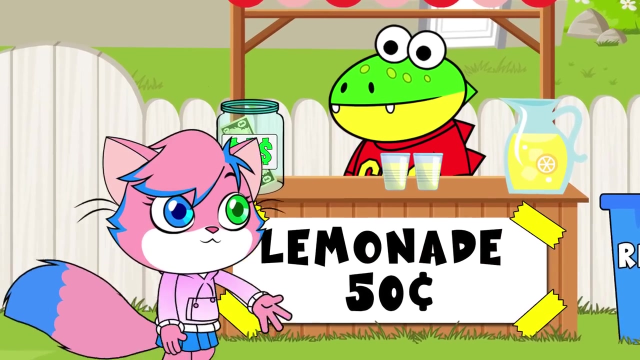 Because each quarter equals 25 cents, And 25 plus 25 is 50!. There you go, Shug. Here's your change, Gil: 50 cents. Thanks, dude, Ah, Ah, Just when I need it. Hey Gus, Could I have two cups of lemonade please? 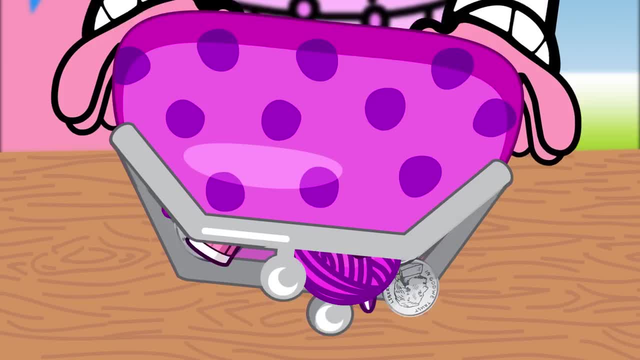 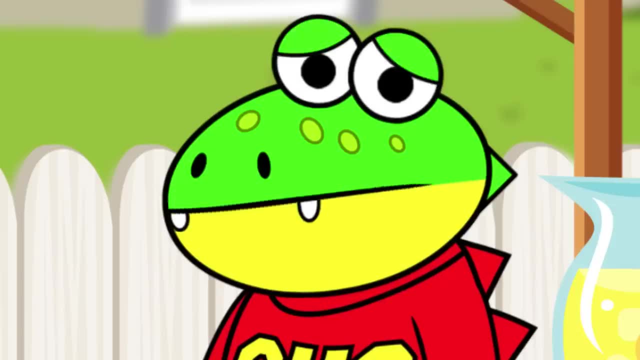 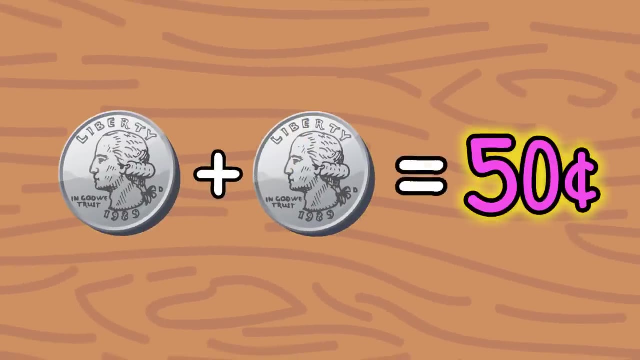 Sure thing, Alpha, That'll be one dollar. please. Sorry for all the coins, but I think you can figure it out. Uh, okay, So it looks like you have two quarters here, which is 50 cents. Now you just need 50 more cents. 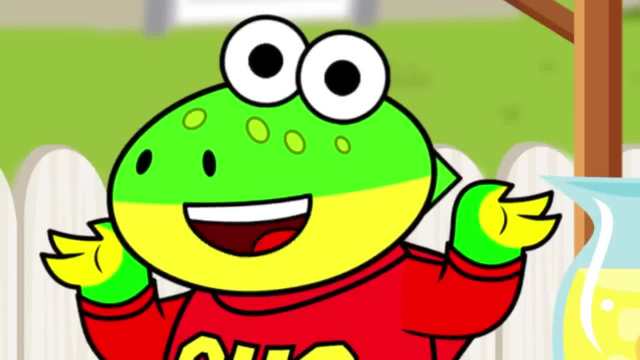 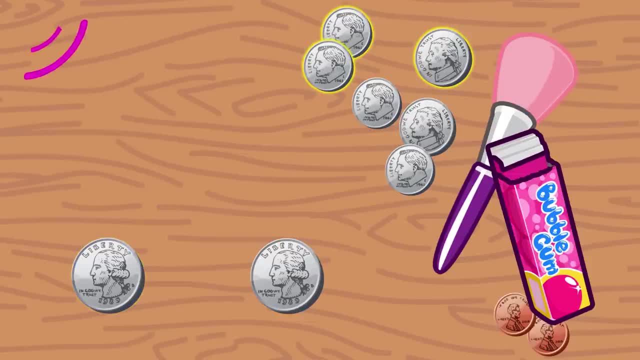 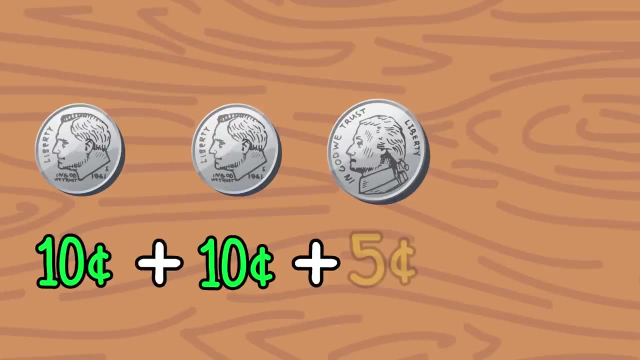 What coins should I use to make another 50 cents? Little Gators, Two dimes and one nickel equal one quarter Gus. So double that. Oh, Good thinking. Little Gators, Two dimes and one nickel do equal one quarter, which is 25 cents. 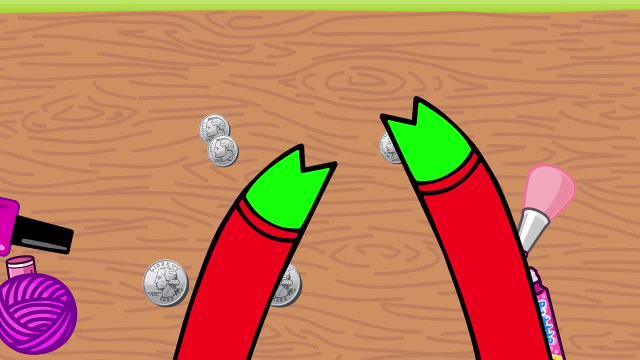 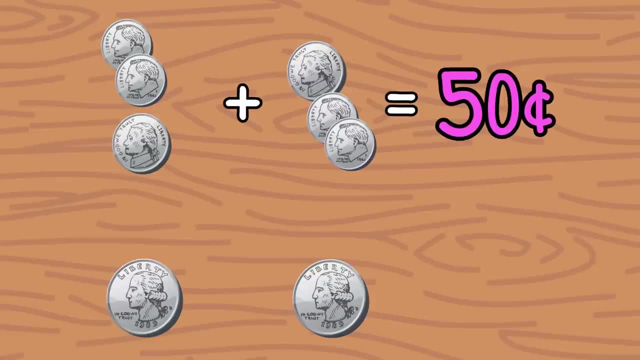 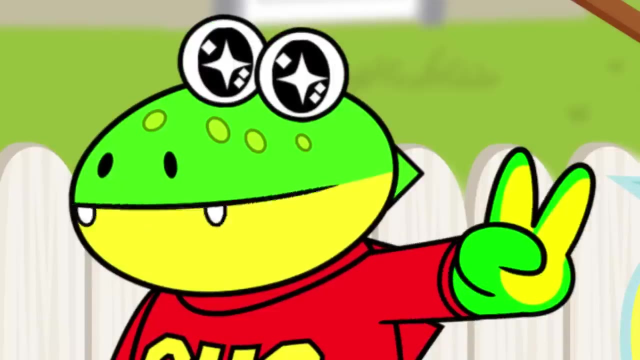 So if I do that two times, I will have four dimes and two nickels. That equals 50 cents. Now we have 100 cents, and that equals a dollar. Thanks for your help. Little Gators, Looks like you've got it covered. Alpha, Here are your two cups of lemonade. 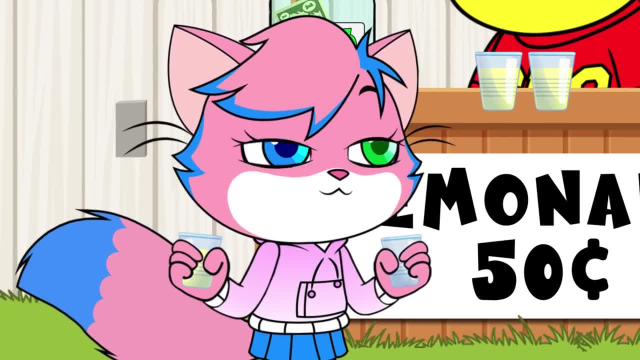 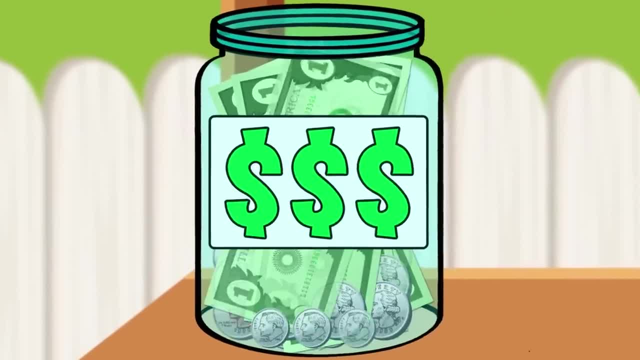 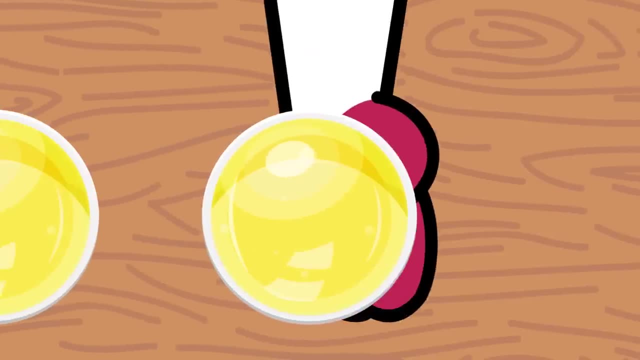 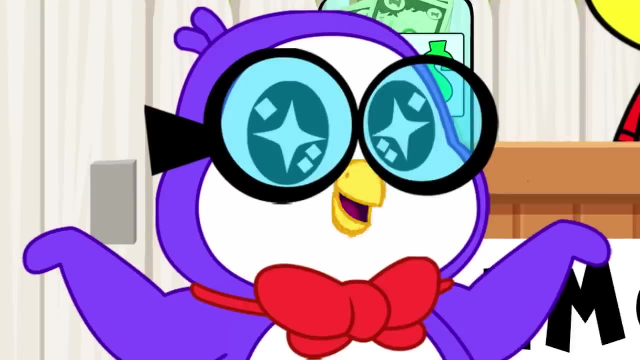 Wow, This lemonade is purrrrrfect. Thanks Gus. Hey Gus, You got quite the business going. Do you have any more of this pecktacular lemonade I've been hearing about? Sure, do Peck, That'll be 50 cents. 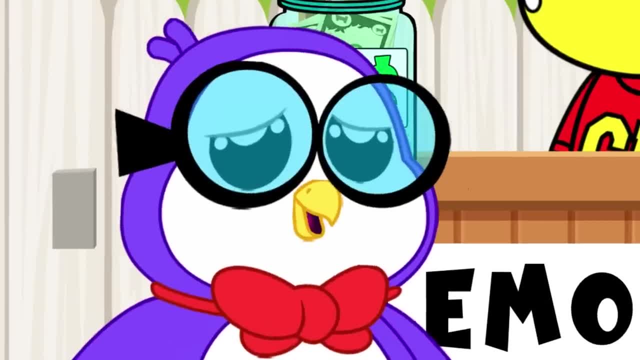 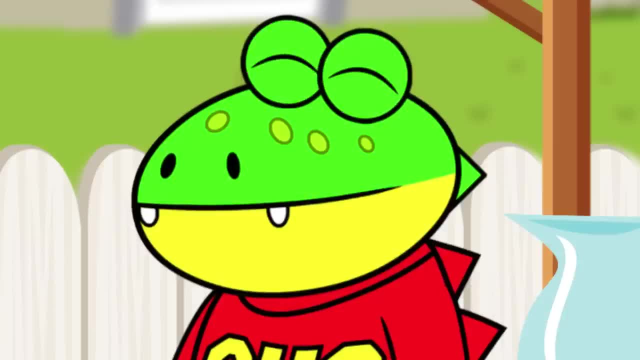 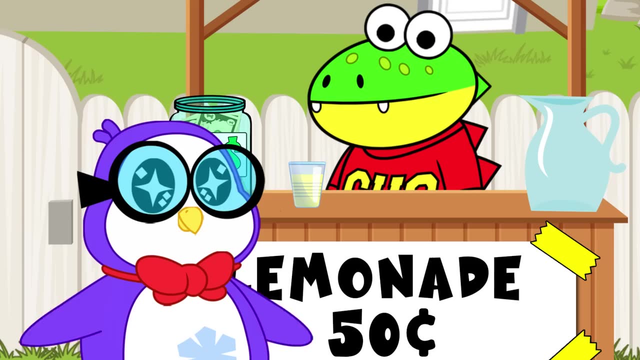 Uh, uh, Oh, Oh no, I must have left my money at home. I guess I'll have to try the lemonade another time. No worries, Peck Here you go On the house, Really. Oh, thank you, Popsicles on me next time. 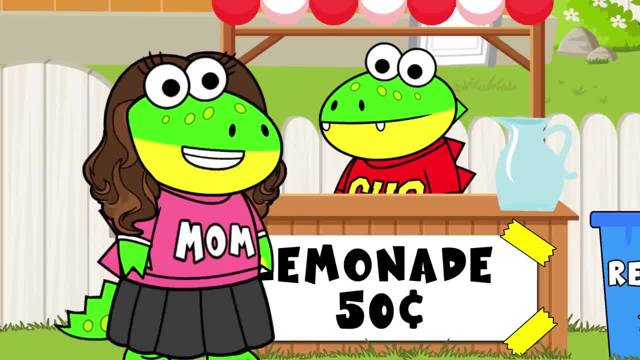 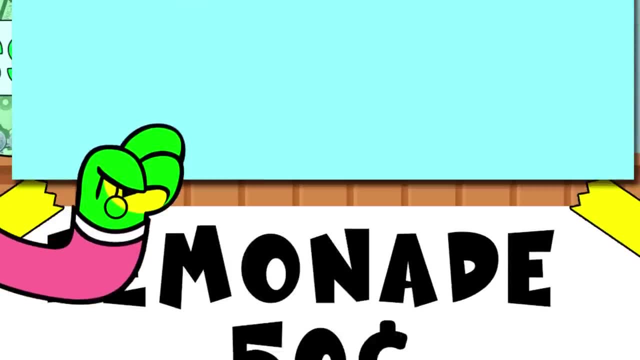 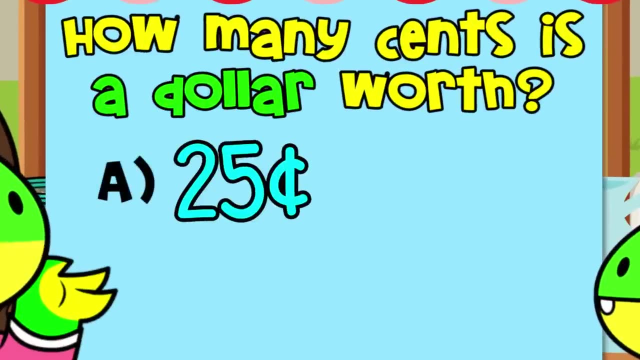 Wow, Suge. Looks like you had quite the turnout today. Sure did Mama Pop quiz Gus. Let's see what you learned. First question: How many cents is a dollar worth? A 25 cents, B- 75 cents. 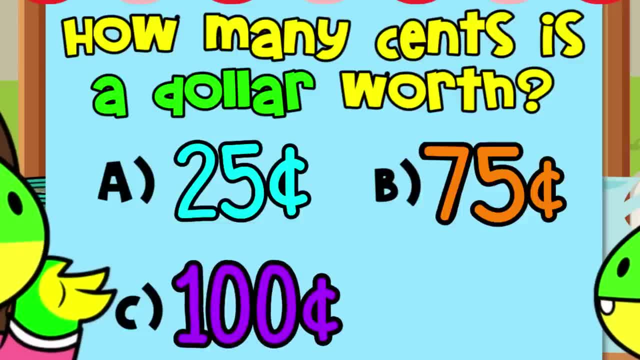 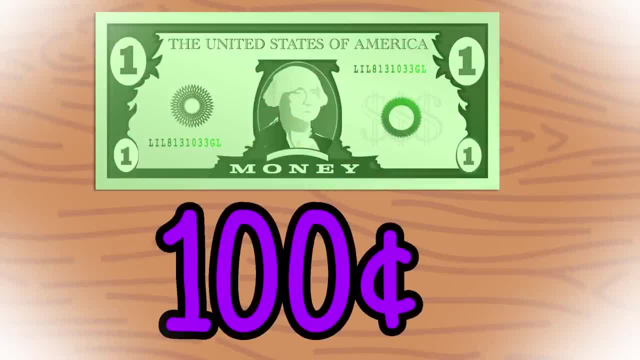 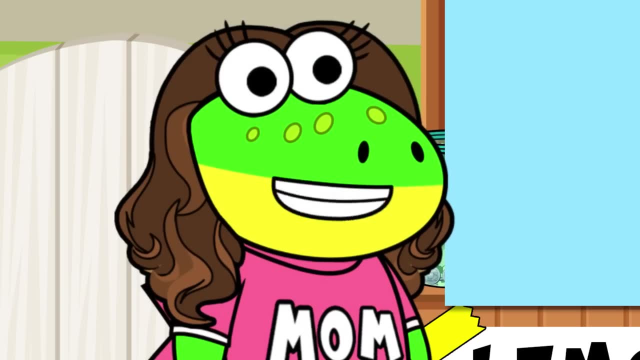 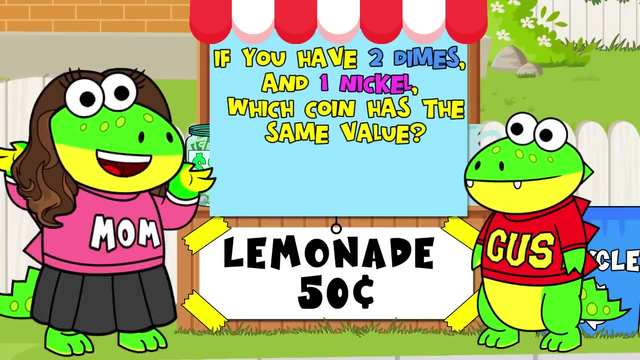 C 100 cents Or D 50 cents. A dollar equals 100 cents. The answer is C 100 cents. Good. Next question: If you have two dimes and one nickel, which coin has the same value? A A quarter.